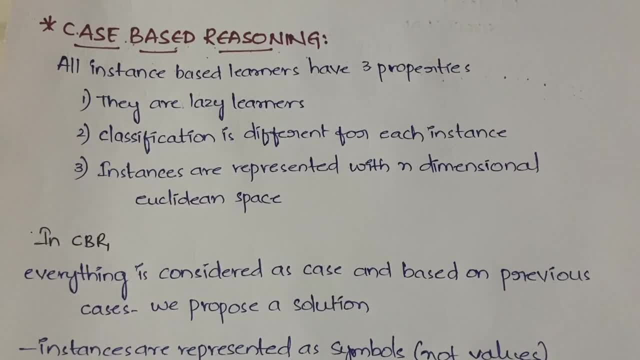 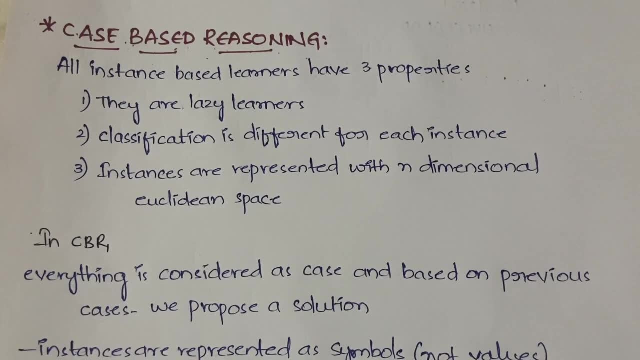 total of three, and among that we have learnt about already two: the lazy learners and the radial-based functions. So in this video we are going to learn about the case-based reasoning. okay, done, And if you are having your exams scheduled nearby, just let me know. 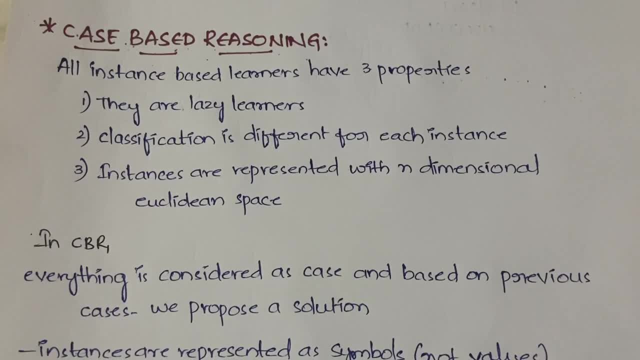 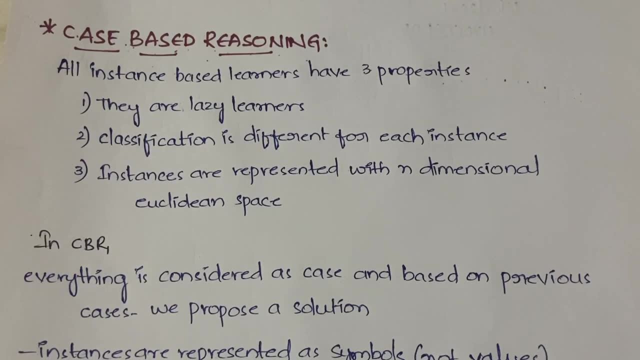 the date of your exam in the comment section so that I can make videos quickly by your exam date. And yeah, let's get into the video now. So first, before learning what case-based learning is, we have to understand what are the properties of instance-based learning. 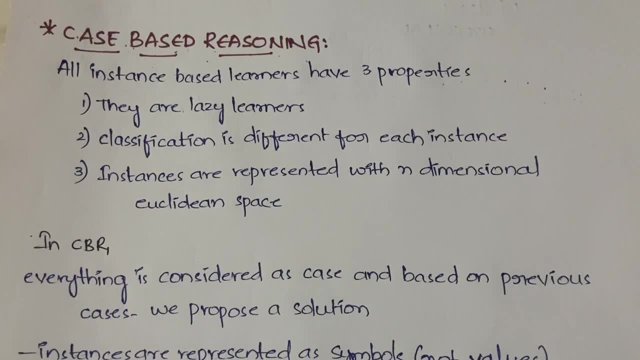 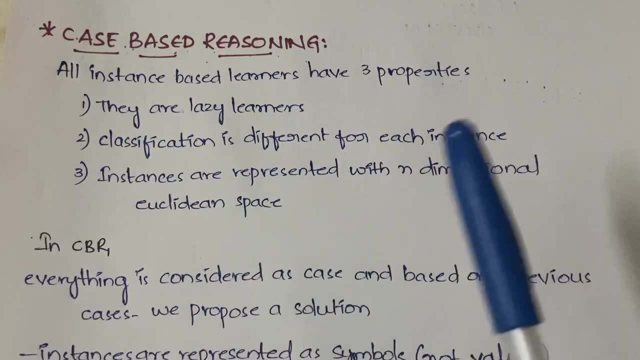 okay, So instance-based learners actually have three properties. They are the lazy learners, the classification is different for each and every instance, and instances are represented with n-dimensional Euclidean spaces. So these are the three properties We have associated with the instance-based learning. So, from these three properties, 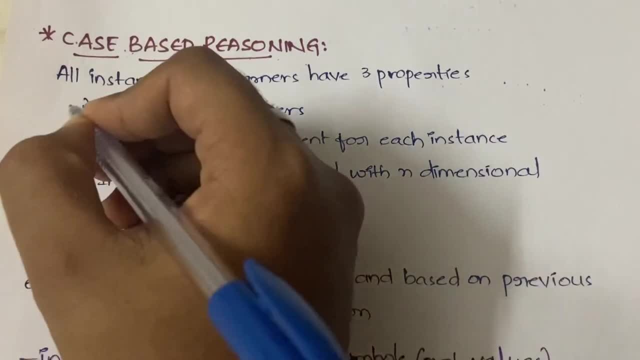 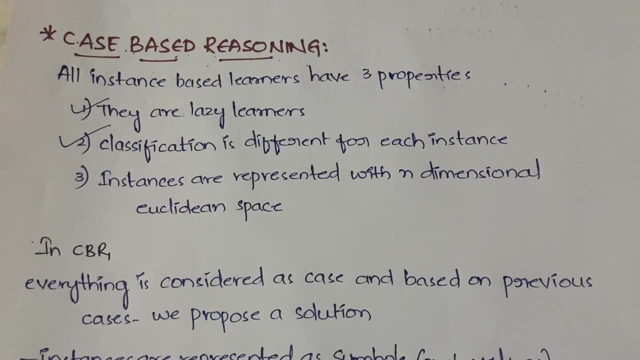 the case-based reasoning follows the first two properties. okay, They are the lazy learners, and classification is different for each instance, So the case-based reasoning is mainly depending on these two properties. okay, done. So how case-based reasoning is actually done and 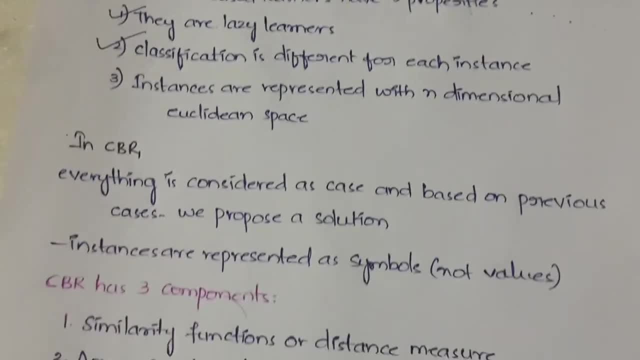 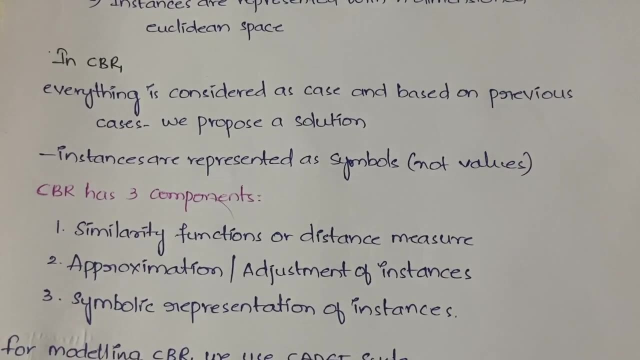 I will explain you this with an example as well, don't worry, okay, done So in case-based reasoning. everything is considered as a case, So every you know what is the case, right, in which case we use case statement: case 1,, case 2, case 3, that is. 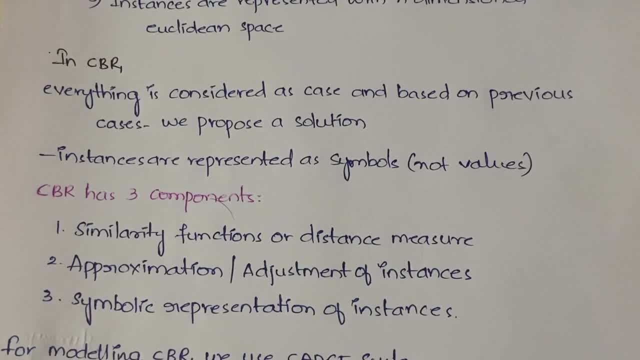 situation 1, situation 2, situation 3, like that. So based on which situation, how it will react. So in the same way, everything is considered as one case and based on the previous cases, we propose a solution. So previous, identical case, based on the previous identical situation. 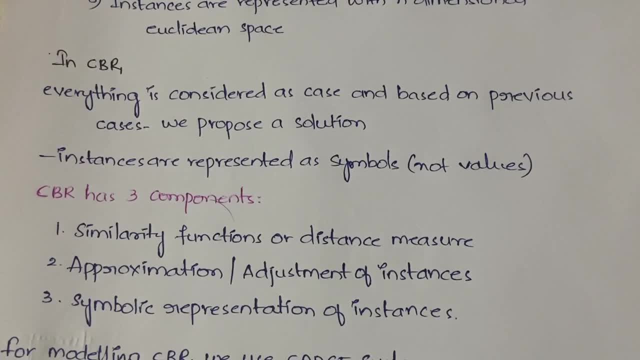 like this: we will be giving a solution. okay, You will understand it more clearly with an example, don't worry. So when I go with example then you can understand it more clearly. Now see, in case-based reasoning we actually have three components, and before that, in case-based 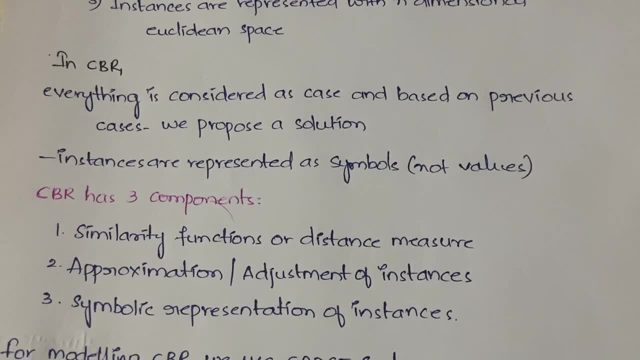 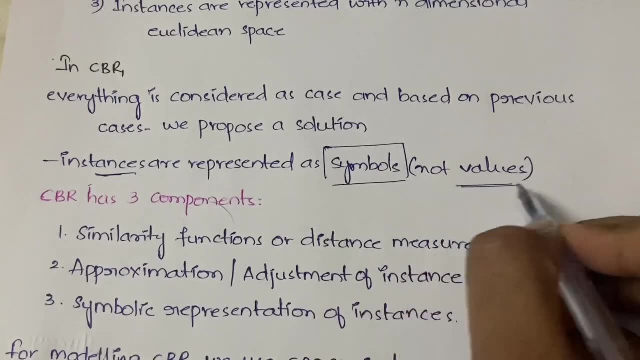 reasoning in every machine learning algorithm will have instances, right. So here, in case of case-based reasoning, these instances are represented in terms of symbols, not values, not real values or continuous values or nothing, not in terms of any type of value. they are. 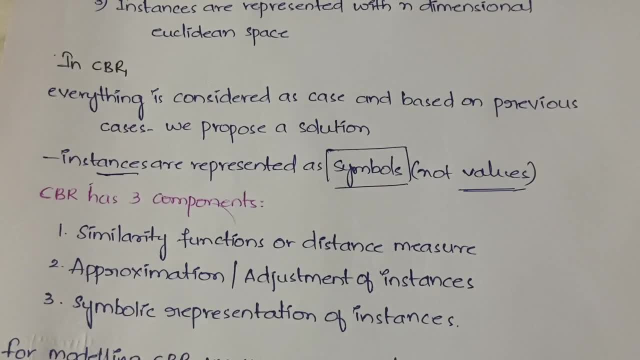 represented only in terms of symbols. okay, Are you getting it? So instances are always represented with the help of symbols in case of case-based reasoning. So in case-based reasoning, case-based reasoning. So here, in case-based reasoning, we are actually having three components. 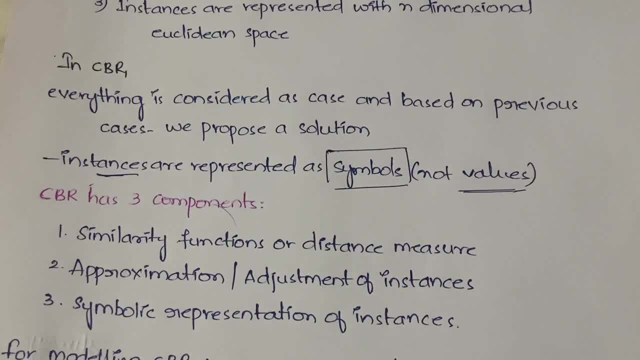 okay, They are similarity functions or distance measure. the second is approximation or adjustment of instances and the third is the symbolic representation of instances. okay, So these are the three components we have in case-based reasoning. okay, Done Now for modeling a case-based 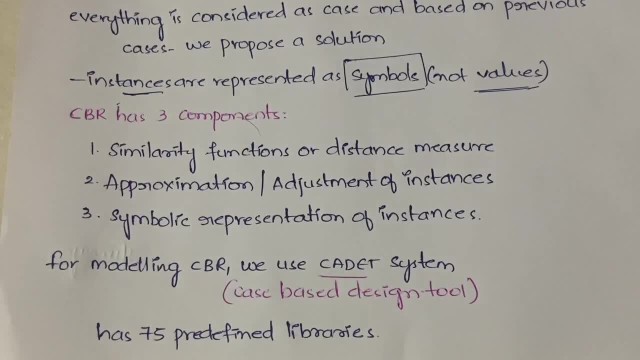 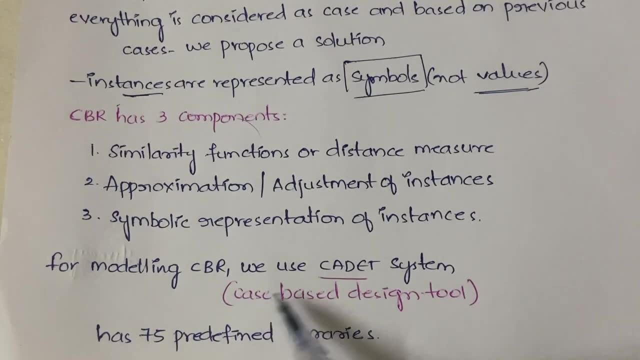 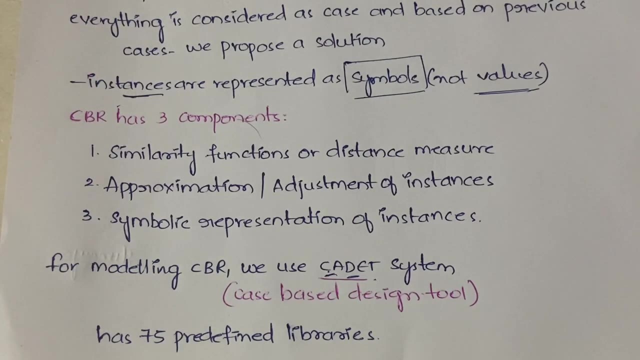 reasoning system. so for modeling a CBR case-based reasoning, we will be using a system which is ADET, CADET system. CADET system stands for case-based design, case-based design tool. okay, case-based design tool. So, based on this design tool, we are going to model the case-based reasoning. 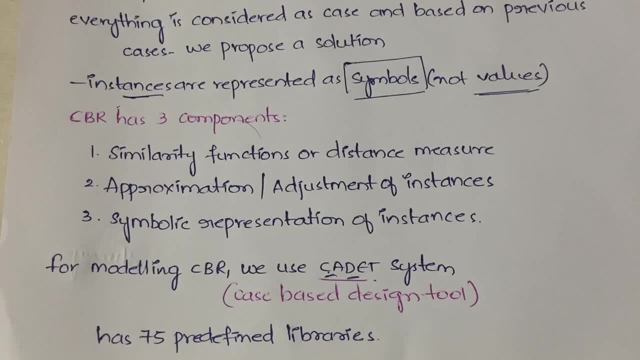 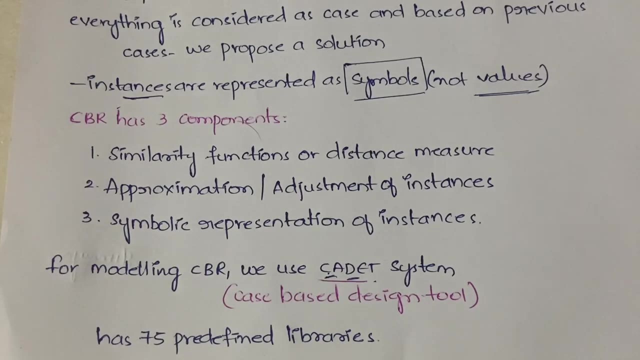 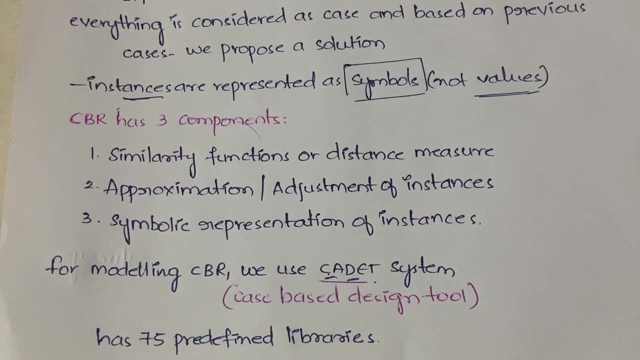 So here, in this case-based design tool, in this CADET system, we already have 75 predefined libraries. okay, You know what predefined are and what user defined are right. So we already have 75 predefined libraries. So, using these 75 predefined libraries, we will be generating any new things we want to generate. If we want to generate any new situations or any new cases or any new solutions, then we will be doing that with the help of these 75 predefined libraries. okay, Now, for example, as I told, I will explain you with an example so that you can understand it more better. So, for example, let us take an example of modern water taps. okay, So in modern water taps, 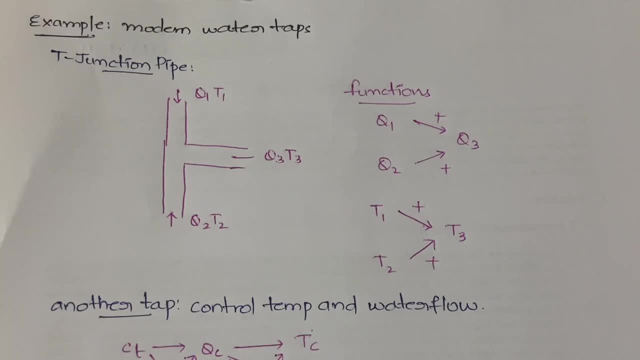 you will have a T kind of T junction kind of thing. right. When you lift up the tap, the water will come, and when you turn the tap to the left side you get hot water, and when you turn it to right side you get cold water and all. and if the tap is in the middle you will be getting a combo of both hot water and cold water. That is a modern system we see in our houses nowadays, right, So previously it was like you know, you need to turn, So previously we do not have any hot water taps. actually no gazers. right. Then gazers came into picture. Then 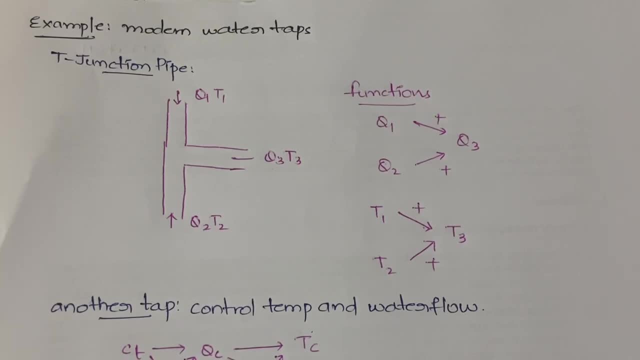 hot water tap, two separate hot water tap and cold water tap, or again, after a few days, the wall mixture came into picture like that. So the evolutions keep on coming right. So here we are, taking the example of a T junction tap, where you lift the tap and you will be getting the water and, based on the direction of the tap, if it is complete towards left side, you will be getting hot water. if it is complete towards So that tap, let us consider, okay Now, so in our example, so, as I already said, in case-based reason, 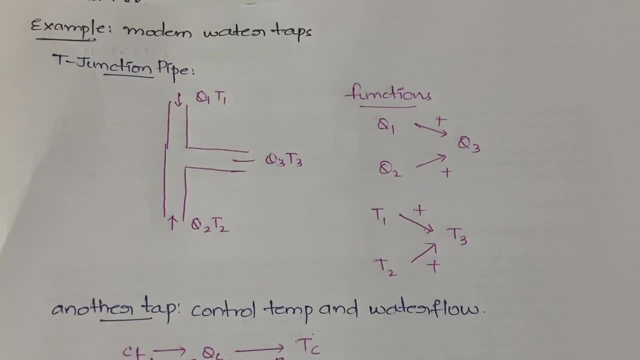 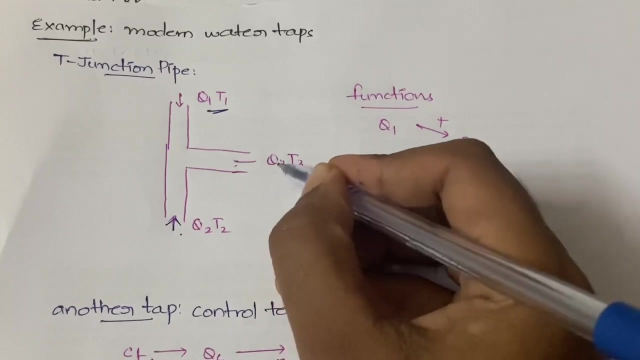 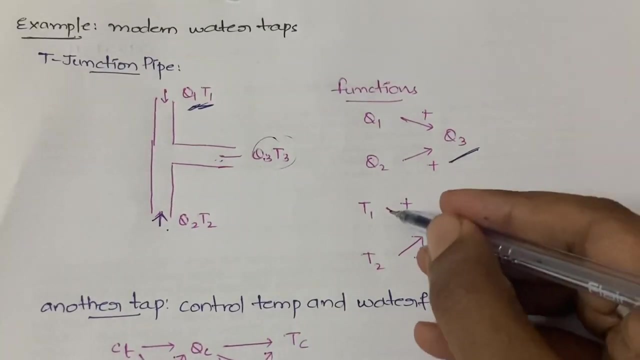 we use symbols. We do not use any values, right? We use all symbols only. We represent it with the help of symbols only. So here, Q means water flow and T means temperature. okay, So here it is Q1 and T1, and from here it is Q2 and T2, and here it is Q3 and T3, which is a combo of both Q1, T1 plus Q2, T2.. See, Q1 and Q2 will give you Q3, and T1 and T2 will give you T3. So this is the basic system we have in our house, right? So this 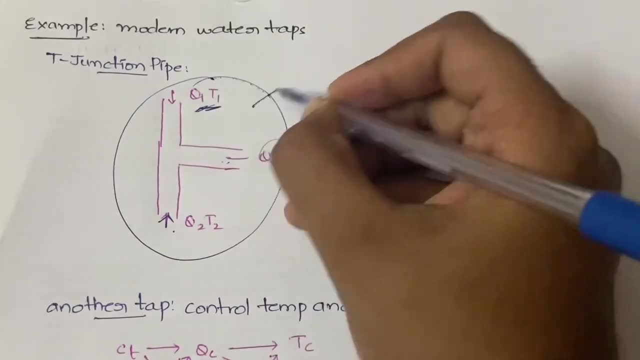 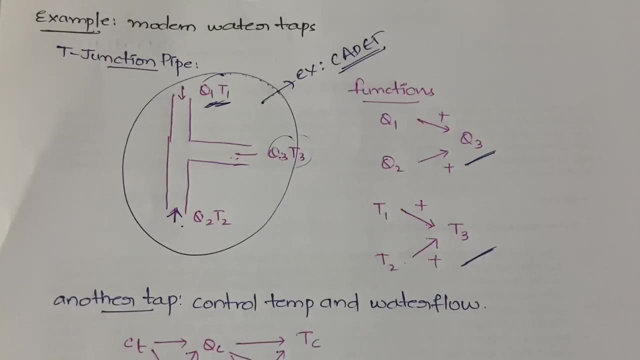 is the already. this is all say: like you know, this kind of example is already defined in CADET system. let us suppose: okay, So CADET. why will CADET system have about taps? do not think like that. I am just giving you an example to understand how case-based reasoning 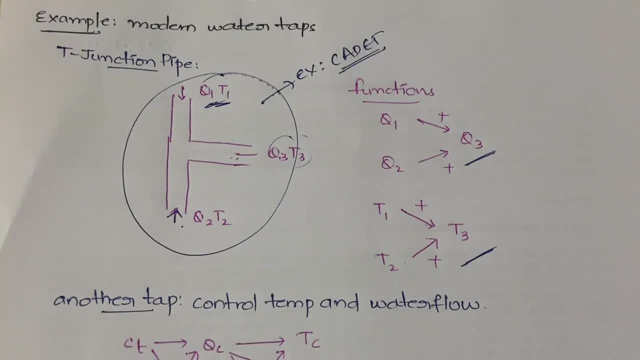 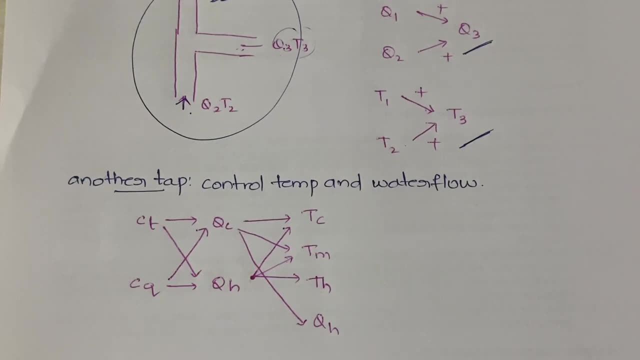 works, okay, Done. Now the requirement is: you need to. you know you need to. you know construct, or you need to manufacture another tap which will control the temperature and water flow. That is you, you can. so in this here, you have only the option to choose either hot water or cold. 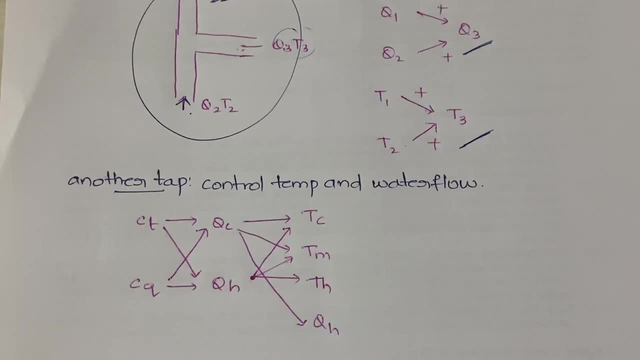 water, but you do not have the option to choose the flow of water, okay. Or you do not have the option to choose the temperature, the range of temperature- either hot or cold, cold, complete hot or complete cold. But here you want a system where you can control the. 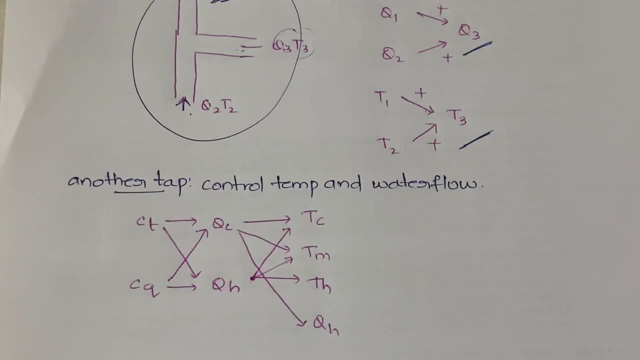 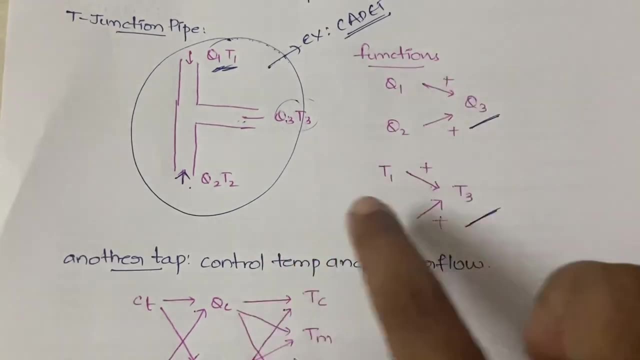 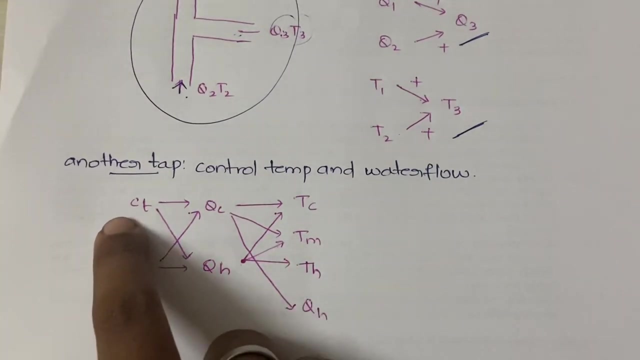 temperature also. So, for that, what you will do, you will be taking the help of this system, which is already existing in the system. You will be taking the help of this and you will be doing some modifications to this system In order to get the system that you have desired. okay, So here, C stands for the control.